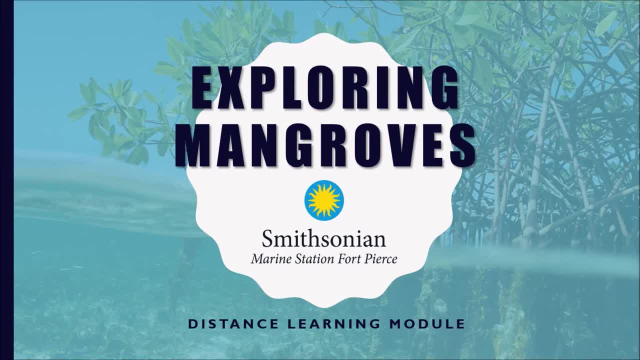 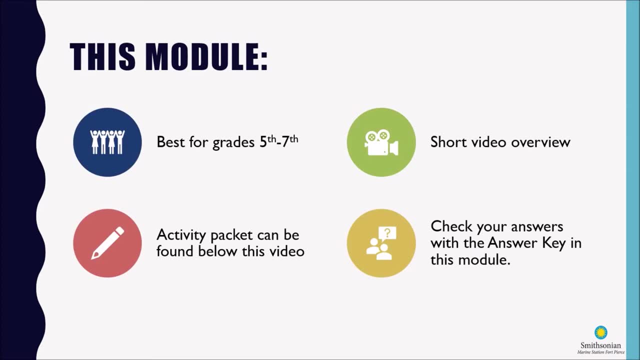 at the Aquarium. Our contact information will be at the end of this video, So this module is best for grades five through seven. We're going to start with a short video overview. As I said, the activity packet can be found below this video and 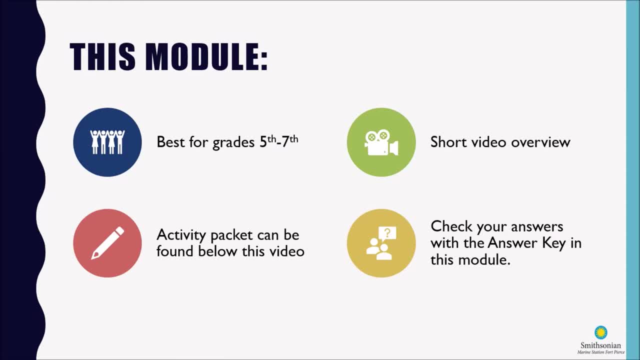 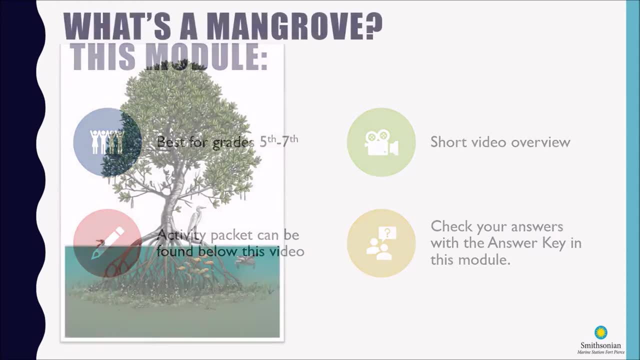 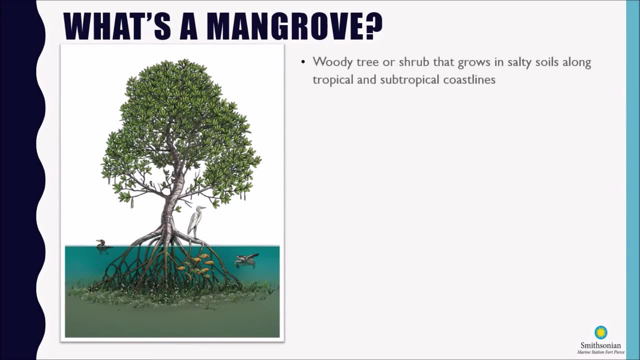 once you're finished, you can check your answers with the answer key, which is also included in this module. Okay, well, let's go ahead and get started. So what is a mangrove? A mangrove is a woody tree or shrub that grows within reach of the 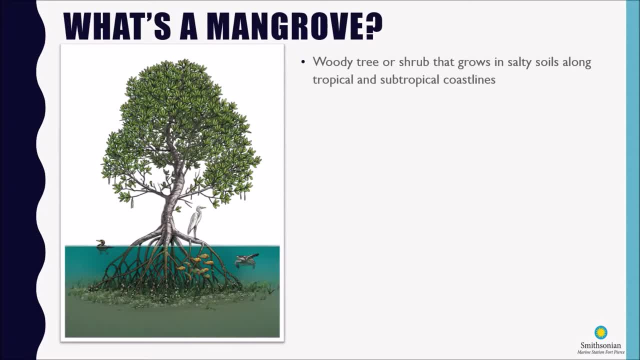 tides in salty soil along tropical and subtropical coastlines around the world. We find 54 true species of mangroves worldwide. That includes the three species of true mangroves that we find here in Florida. We'll talk a little bit more about that in just a minute And it's important to note that mangrove 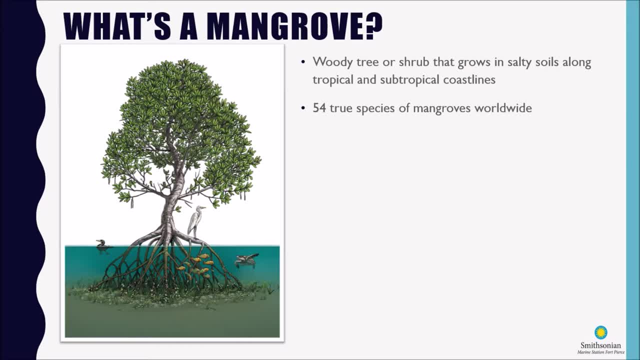 species are not necessarily closely related to each other, but they're classified as mangroves because they all share some common characteristics. So what makes a mangrove a mangrove? Well, first, they are adapted to live in and directly next to saltwater. 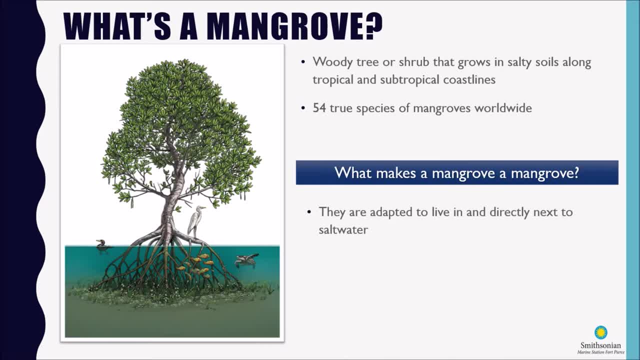 water. Now this can include brackish water areas as well, And remember that brackish water is kind of a mixture of saltwater and freshwater, So brackish water is not quite as salty as saltwater, but it's saltier than freshwater. It's a mixture of the two. 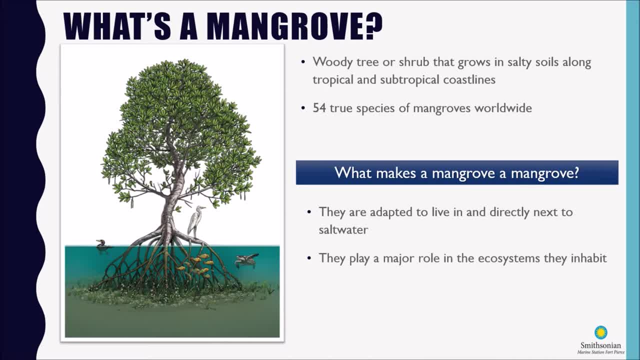 Mangroves also play a major role in the ecosystems they inhabit. We'll talk a little bit more about that as we go forward. And also, mangroves are biologically different from trees that can only survive on dry land, And that's because mangroves have some special 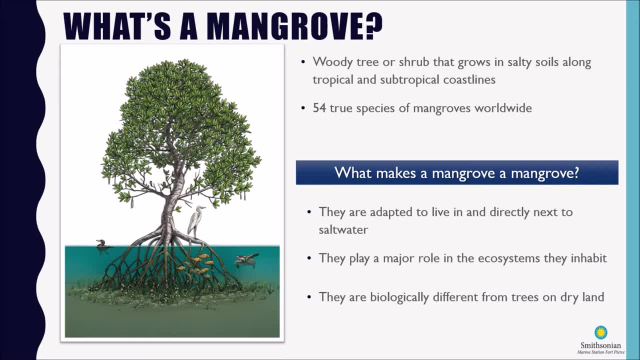 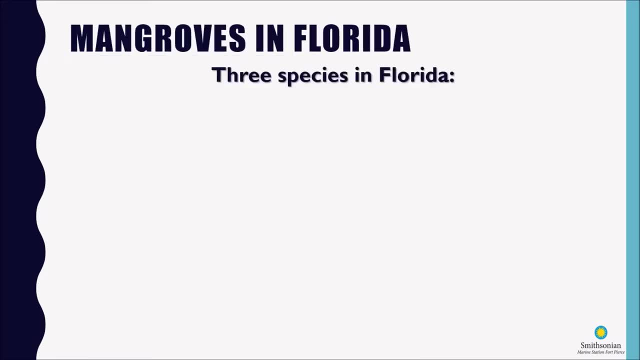 adaptations that allow them to grow in the areas that we find them, And again, we'll explore that a little bit more as we go forward. So let's talk about the mangrove species that we find here in Florida. Probably the most recognizable is the red mangrove- Red mangroves- 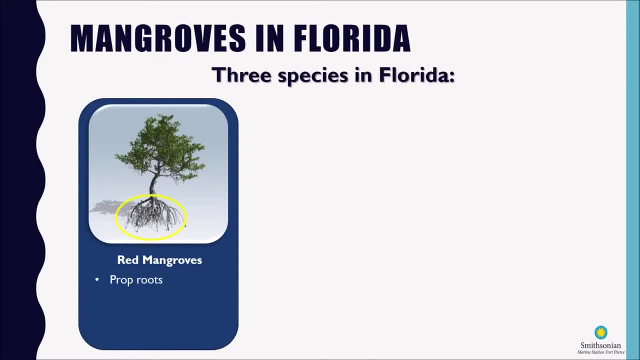 are pretty easy to identify by their prop roots. So prop roots is a root system that props the roots to the soil And it's a system that props the roots to the soil And it's a tree up out of the water. It provides stability for the tree And it allows the roots to obtain. 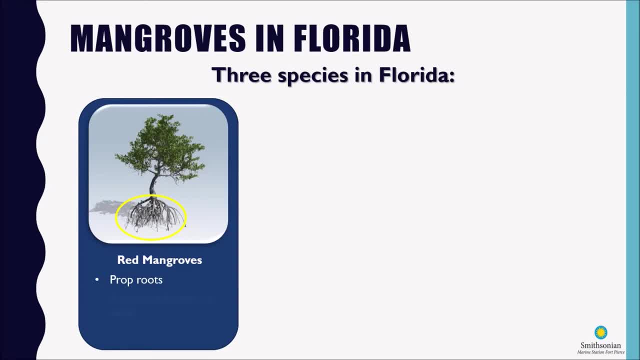 oxygen from the air. Red mangroves always grow along saltwater or brackish coastlines, in either the water or in the mud or the sand. You might sometimes hear red mangroves referred to as walking trees, since it looks like it's walking across the water And red mangroves. 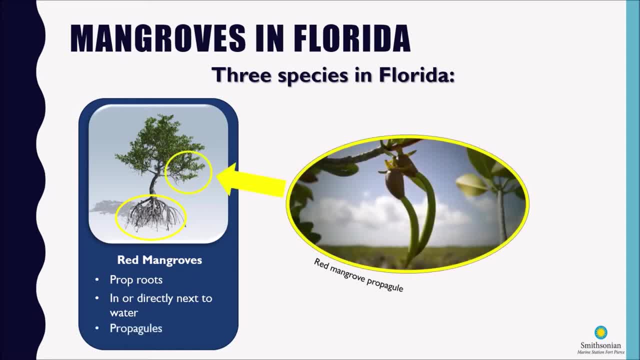 produce something called a propagule, And here's a picture of them right there. Now. this looks like a seed pod. However, propagules are actually living trees. When the propagule falls off of the parent mangrove tree, it can float in the water for up to a year- maybe a little bit longer- before taking root. Another 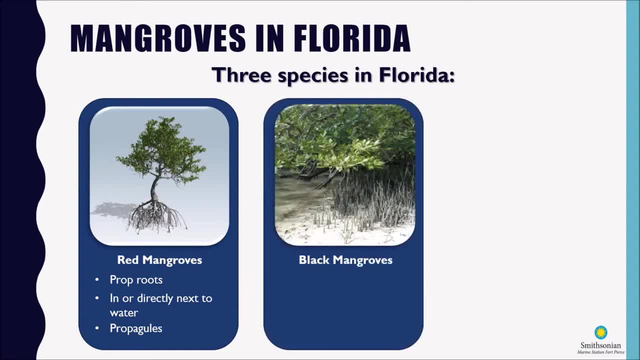 species that we see commonly in Florida are the black mangroves, And black mangroves usually grow either directly or indirectly, But the mangroves that we see in Florida are the black mangroves, And black mangroves usually grow either directly or indirectly, And so they're. 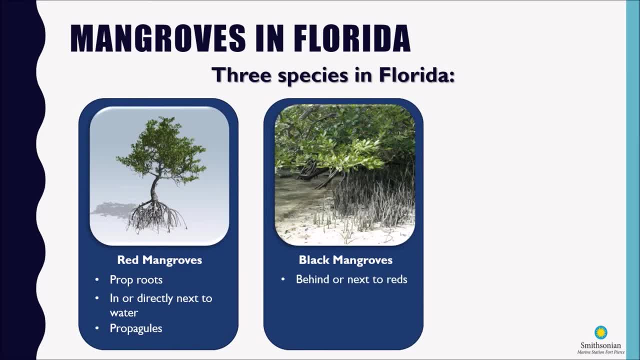 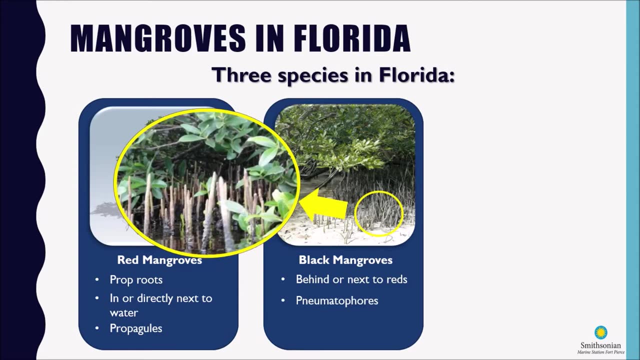 either directly behind red mangroves or very close to them along the shoreline, And they're also easy to identify by their root systems. They have roots that are called pneumatophores, And there's kind of a close-up picture of pneumatophores of a black mangrove tree. These 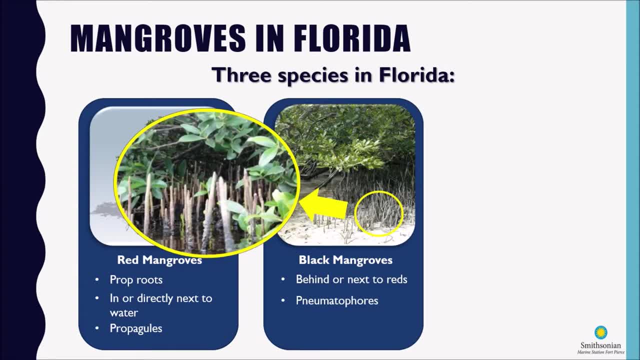 are specialized roots that grow upwards. They grow out of the bottom and up through the water or the mud to reach the air and to provide oxygen for the root system, And the mangrove tree is one of the most common root systems in Florida. This is because the substrate that we 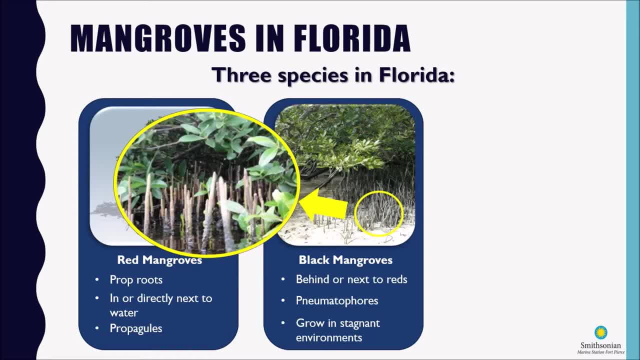 find them in and in red mangroves as well. they tend to be substrates that might be oxygen-poor, so sand mud substrates like that tend to be sort of stagnant without a whole lot of oxygen, So those root systems need to have adaptations in order to get oxygen to their roots. Now white mangroves. 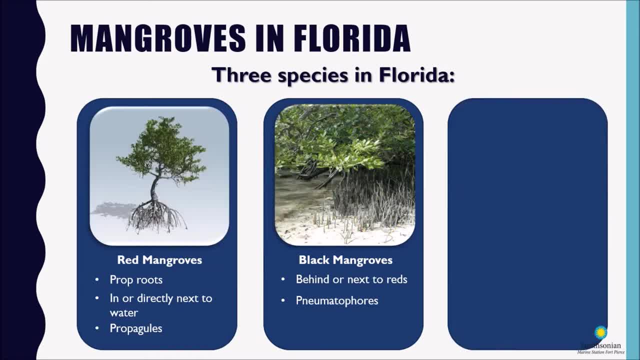 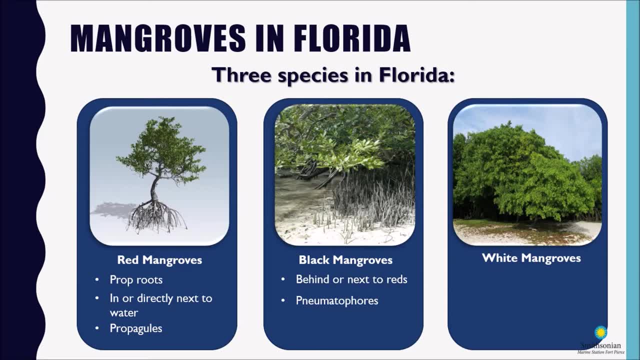 have a little bit of a mixture of brick and mortar. This is a particular example of one of the Now white mangroves can be a little bit trickier to identify. We tend to find white mangroves growing a little further back from the water in an area. 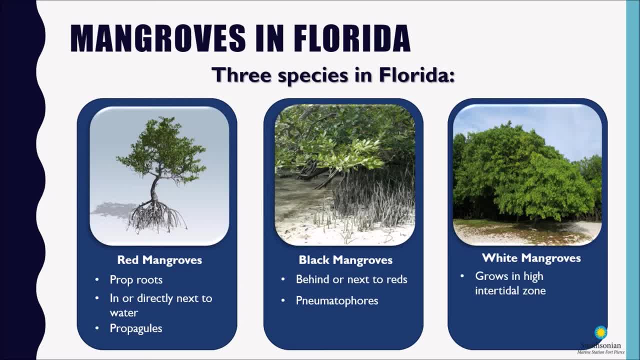 that we call the high intertidal zone. So these are areas that really high tides can reach, like the high tides that we get in the springtime that tend to be higher than during the rest of the year, But it's mostly dry in between those really high tides. 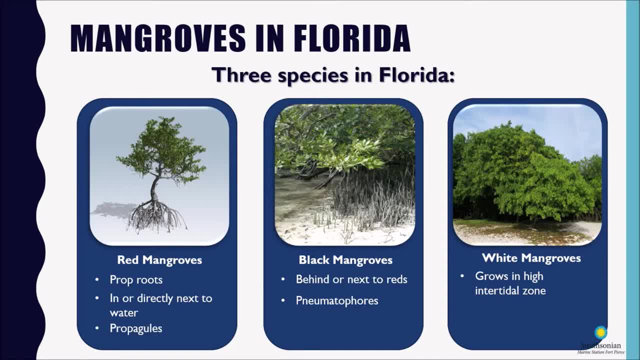 In Florida, we have two high tides and two low tides every day, roughly just over six hours apart. And when I'm talking about tides, remember I'm referring to the regular rising and falling of the ocean due to the gravitational pull of the moon and the sun. 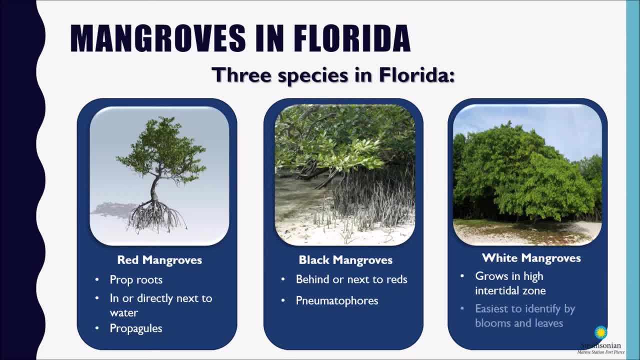 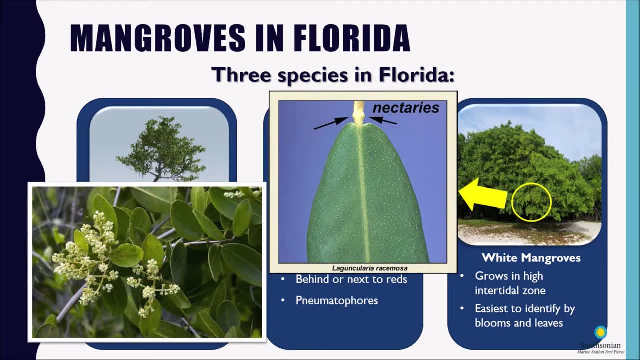 So the easiest way to identify white mangroves is through their leaves And their blooms. So their leaves tend to be more rounded in shape than a red or black mangrove leaf, And they have small nodules above the leaf called nectaries. 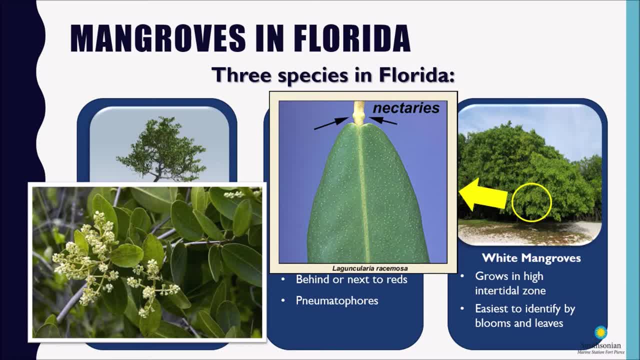 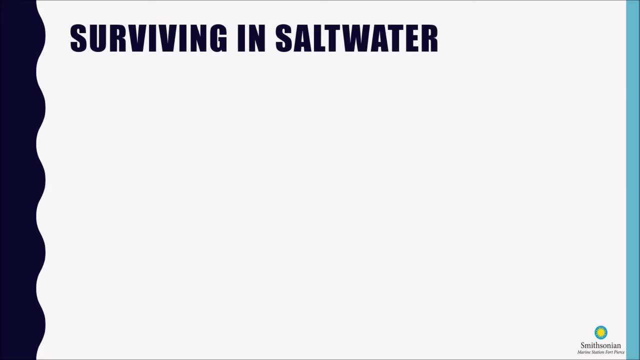 And the blooms that white mangroves produce are kind of delicate white flowers that are really pretty And there's a picture of them right there on the left, So surviving in saltwater. How do trees grow in and around salty water? Do trees need fresh water to live? 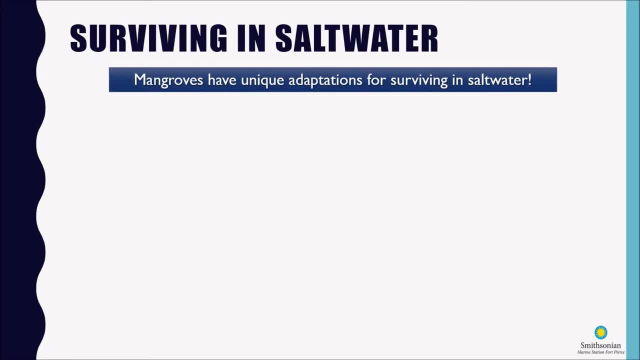 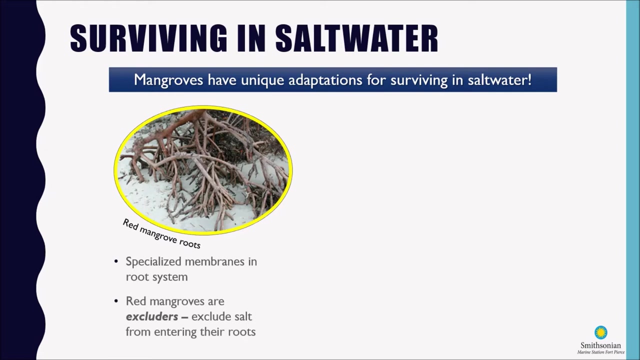 Well, yes, they do, But mangroves have unique adaptations for surviving in saltwater, So red mangroves have specialized membranes in their root systems that prevents up to 90% of salt in saltwater from entering their vascular system. So we call red mangroves excluders, since they exclude salt from entering their roots. 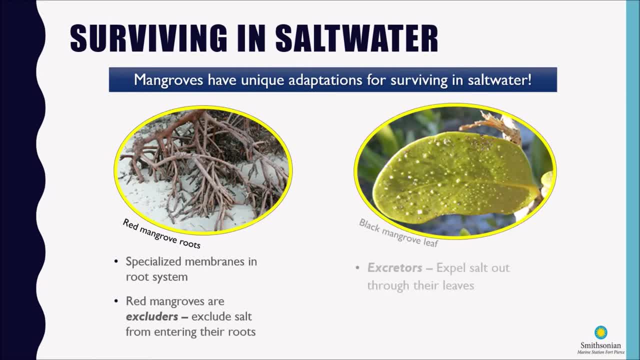 Now black and white mangroves are called excretors because, while these trees can't prevent the uptake of saltwater through their root systems, they'll push salt out through the pores on their leaves, And this is called excretion. Sometimes, if you look really closely on the leaves of the black or white mangrove, you 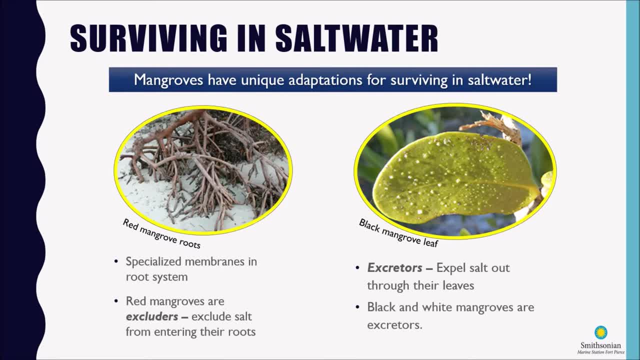 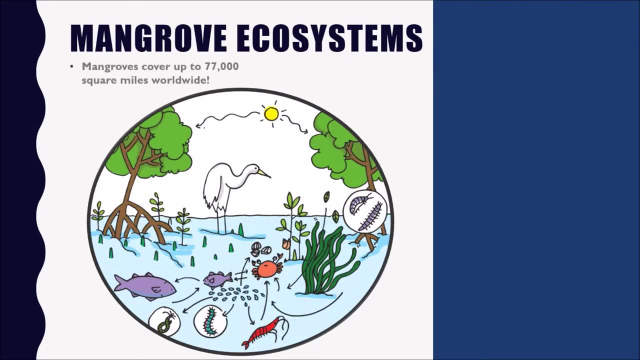 might actually see small salt crystals, like you do in this picture on the right. Okay, All right. So let's talk a little bit about mangrove ecosystems. So, according to the Smithsonian Institution, mangroves cover up to 77,000 square miles. 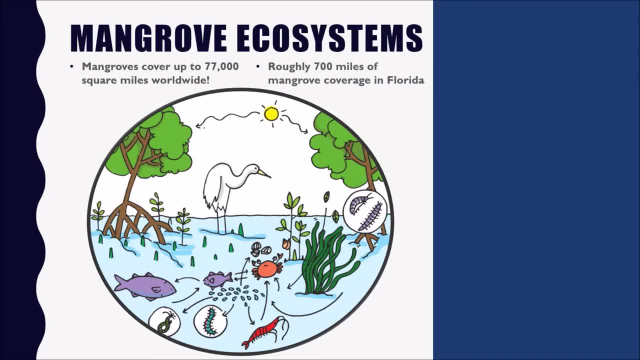 of the earth, And in Florida we have over 700 miles of mangrove coverage, So mangrove forests support a huge diversity of life, either by the animals that consume the leaves, Through animals living in the branches of mangroves, Like mangroves, like nesting birds, and even organisms that live on the roots, like sponges. 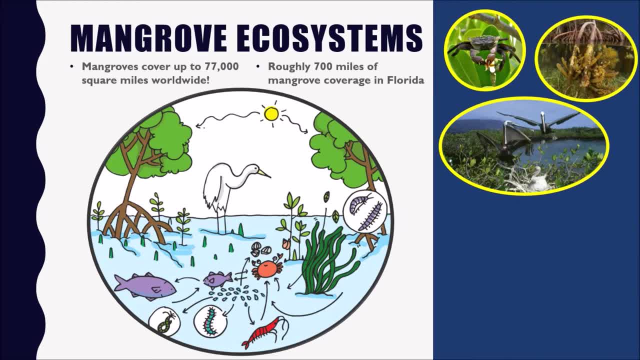 snails, barnacles, oysters and more. So fallen leaves from mangroves are the base of this food web. So mangrove ecosystems are considered to be a detritus-based food web. They support a detritus-based food web. 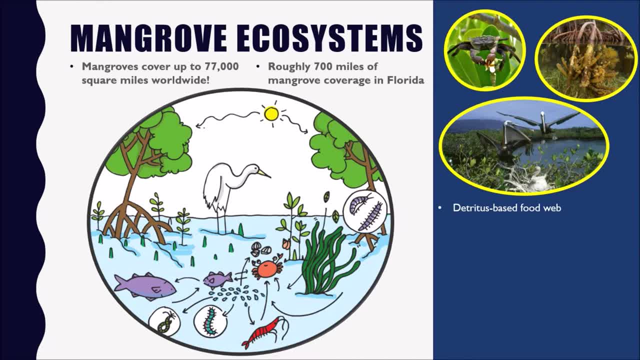 So there are animals that eat the fallen leaves themselves, And these animals are called detritivores Because they consume detritus, which is dead organic material like fallen leaves. Mangrove ecosystems are also considered to be nursery habitats, And that's because we tend to find not only a lot of young animals there that will move. 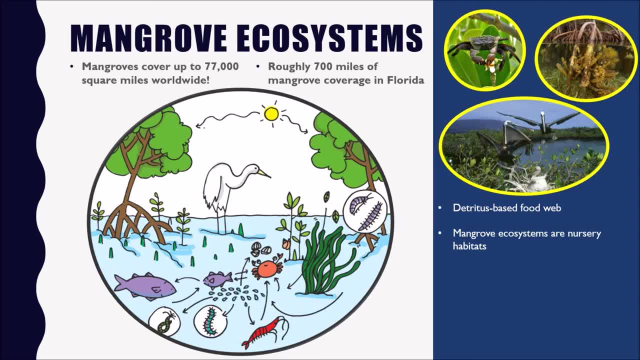 out of that area once they grow a little bit larger, but a lot of these animals only spend part of their lives in those mangrove ecosystems before they move out into deeper water. This would include certain species of shrimp, certain species of crabs and fish as well. 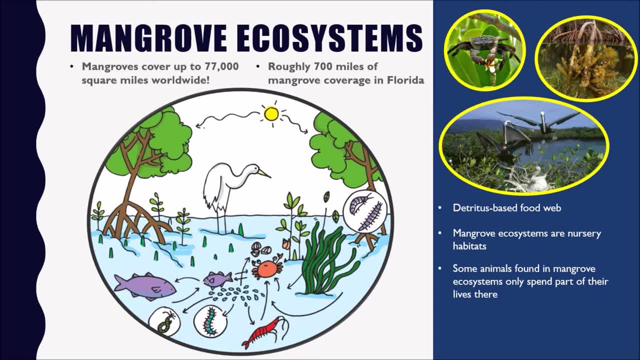 So they'll move out of that ecosystem once they're a little older, bigger and they're ready for deeper water. So even if a bird species does not nest in the branches of the mangroves, many species of birds will use mangrove areas to hunt for food. 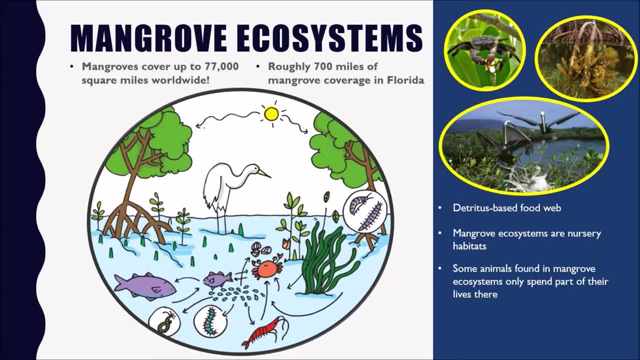 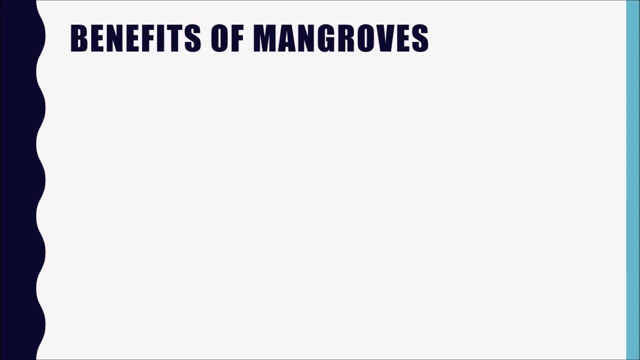 And for swimming species like fish and swimming crabs. the roots of the mangroves are a great place to find food And to also find protection from predators. So there's a lot of benefits to mangroves. There's almost too many to list, so we're just going to hit a few of the most important. 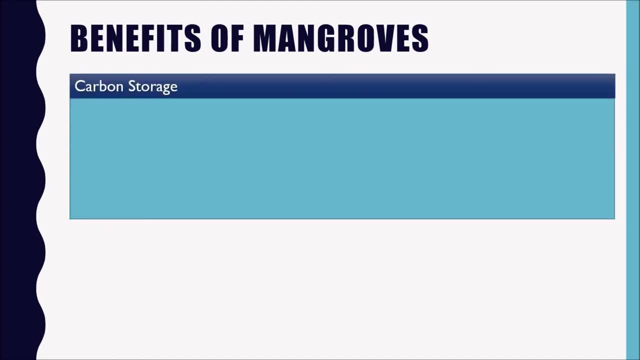 ones, And the first one I want to talk about is carbon storage. So one of the important things that mangroves do for our environment is to absorb and store carbon dioxide from our atmosphere. So carbon dioxide can come from many different sources, Including greenhouse gases. 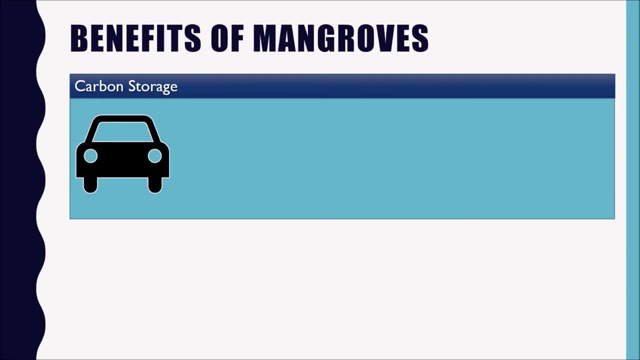 Gases that are produced by fossil fuels, Like gasoline in our cars or our airplanes. And like other plants, mangroves use carbon dioxide from the atmosphere in the process of photosynthesis to build tissues in their leaves, their roots and their trunks. 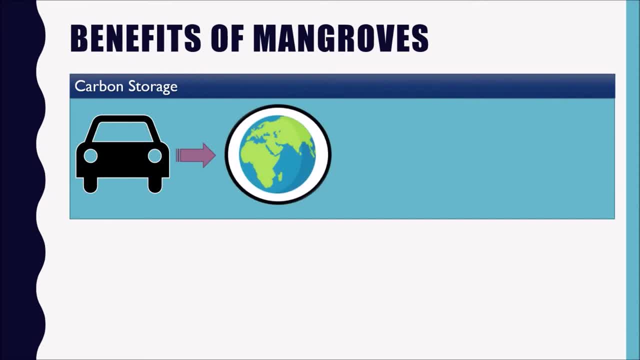 So why is this important? Well, carbon dioxide can trap heat in the atmosphere, And so if there's too much carbon dioxide, then the planet becomes warmer than it should be. Now you may have heard the term global warming or climate change. 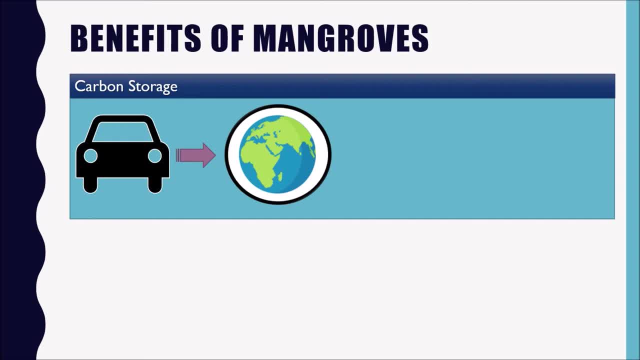 And when the planet is too warm, it can cause a lot of problems. It can cause changes in weather, droughts and the melting of polar ice caps, which leads to rising sea levels. But mangroves can store that carbon and keep it locked away so that it isn't released into. 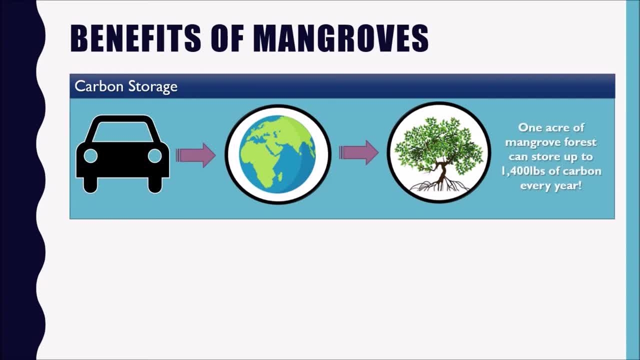 the atmosphere, And one acre of mangrove forest can store up to 100 tons of carbon dioxide, And that's a lot of carbon dioxide, And that's a lot of carbon dioxide. It can store up to 1,400 pounds of carbon every year. 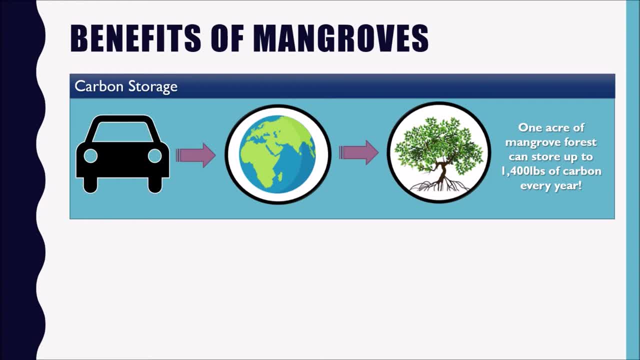 And remember I said that worldwide, over 77,000 square miles are covered by mangroves, So you can imagine how much carbon can be stored from all of those mangroves. Now, mangroves also help to protect our shoreline because they are shore stabilizers. 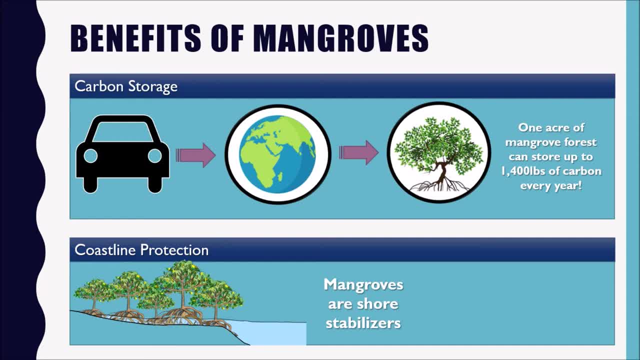 And what this means is that the roots actually help hold the shoreline in place, And what this means is that the roots actually help hold the shoreline in place to prevent erosion. So this is especially important during things like hurricanes, when there are a lot of heavy. 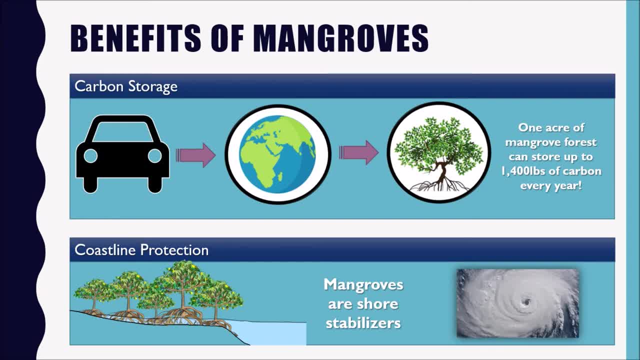 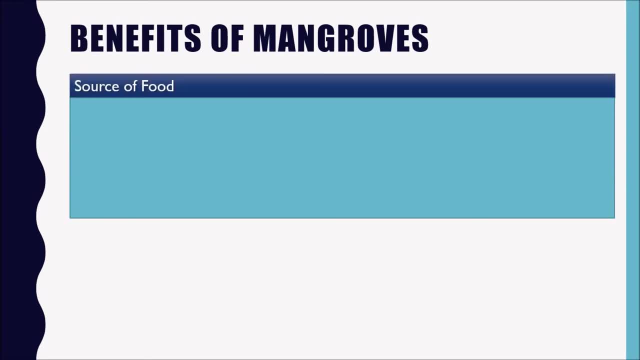 waves and strong winds. Mangroves help to break up the wave energy and to decrease the storm surge. Another benefit is that they are a source of food, and not only a source of food for the animals who are living in those areas, but for us as humans as well. 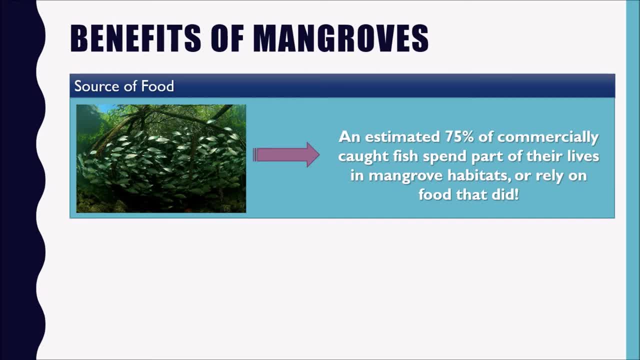 And so mangroves are a source of food for the animals who are living in those areas, but for us as humans as well. And so mangroves are a source of food for the animals who are living in those areas, but for us as humans as well. 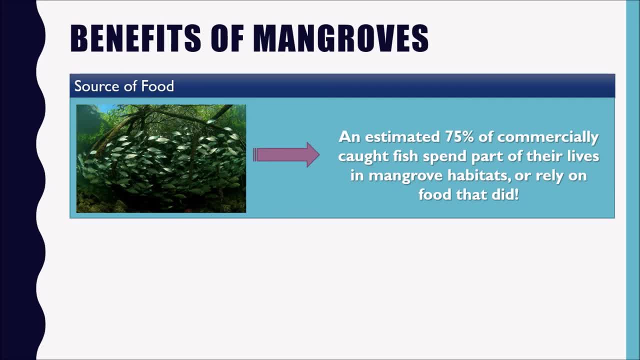 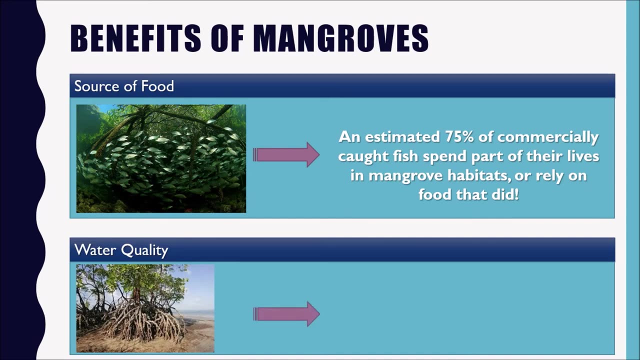 And almost 75% of fish that are caught for food spend part of their lives in mangrove habitats or they rely on food that did. We also rely on mangroves to help us with water quality, So organisms that live on mangrove roots, like oysters, help to filter the water by consuming. 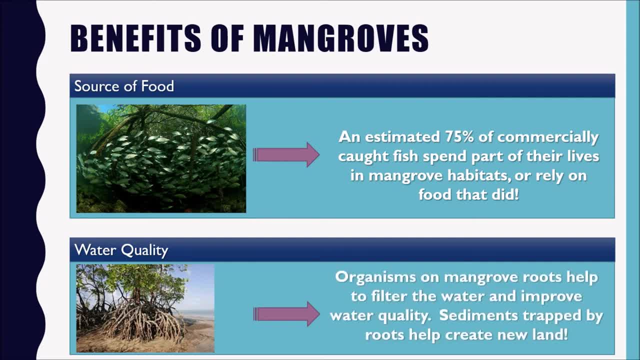 suspended particles in the water, And that can include things like heavy metals or other forms of human-made pollution, And so mangroves are a source of water quality food. They can be used to filter water from water sources, either from land, from water sources. 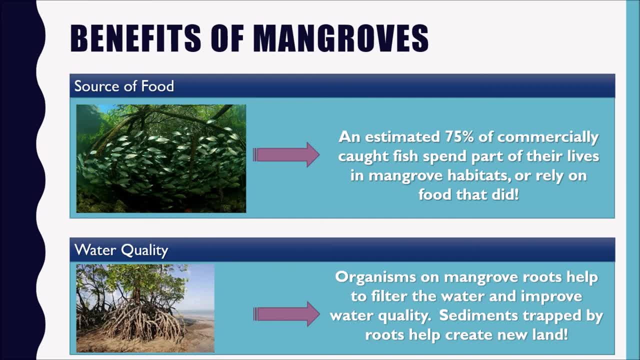 or from other areas of the system, And they can be used to collect heavy metals or other forms of human made pollution or other, And by filtering all of those suspended particles it actually helps increase our water quality. Over time, the sediments that mangroves trap can also become new land. 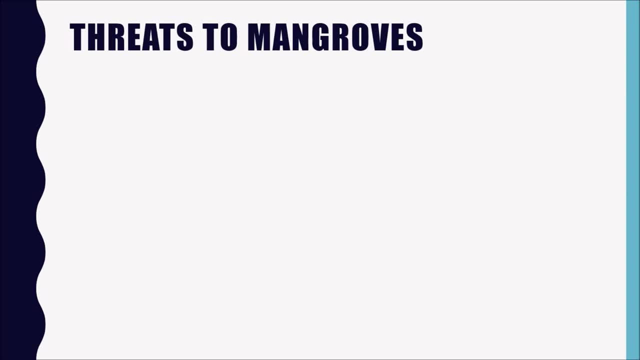 Now, just like there's a lot of benefits to mangroves, there's a lot of threats too. There's a lot of threats to mangroves, So let's just hit a few of them here. The biggest threat to mangroves is actually us. 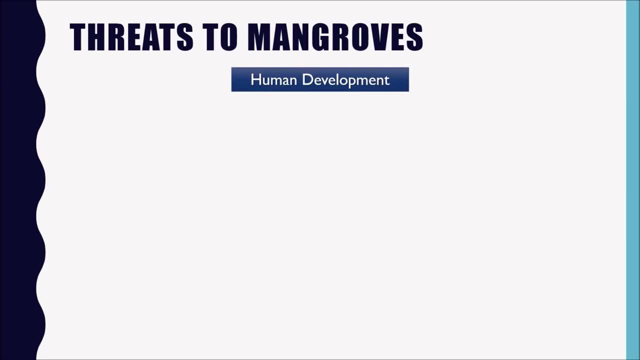 It's humans And that's because humans have removed or destroyed over 6,000 miles of mangrove forests around the world just since 1996.. Sometimes mangroves are removed because humans want to build homes, businesses or other structures in those areas where mangroves are. 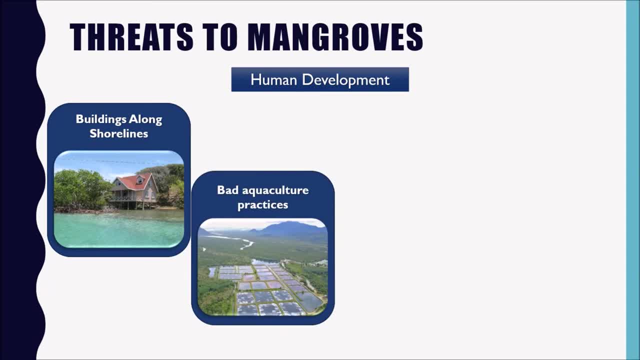 Sometimes, mangroves are removed because humans want to create farms to grow fish or shrimp. This is called aquaculture. Now, aquaculture itself is natural. It's not a bad thing. In fact, it's a very good thing, since we can raise fish and shellfish to eat instead of harvesting them from the wild and contributing to those overfishing issues. 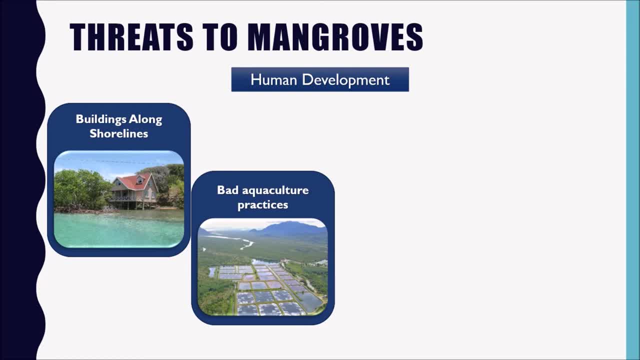 However, there are some countries that practice poor aquaculture techniques that can result in environmental degradation. Now, in other countries, like the United States, strict environmental laws forbid these types of environmentally unfriendly practices. This is true in other countries And we work to protect mangroves. 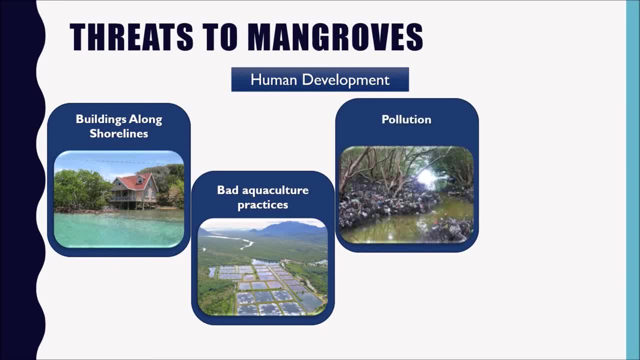 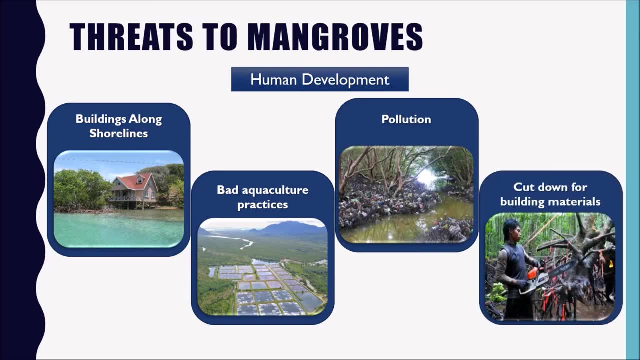 Human pollution can also damage or kill mangroves if the pollution is in the soil, which can keep mangroves from developing and growing properly, And then sometimes mangroves are chopped down in other parts of the world for their wood and used as construction materials. 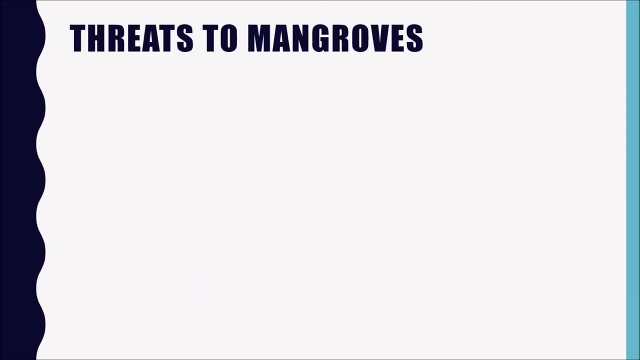 So for houses or bridges, et cetera. Now, although mangroves can actually help us curb some of the effects of climate change, But to expect that they do not, we have to stay away from mangroves, So we have to keep them out of our at-home system. 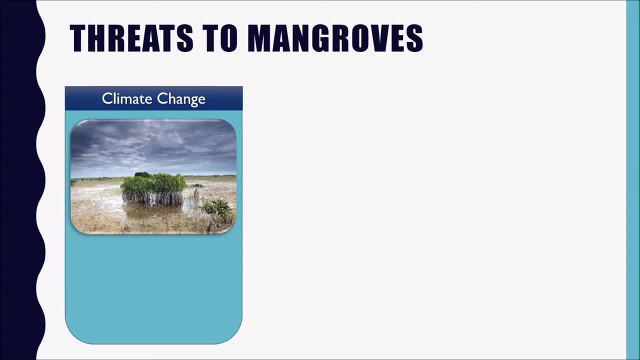 So we have to keep them out of our at-home system And so we have to keep them out of the world. It's very important to protect them from those other elements, So we have to protect them from those other elements as well. change, like we just talked about. mangroves are not immune to it. Okay, So as sea levels rise,